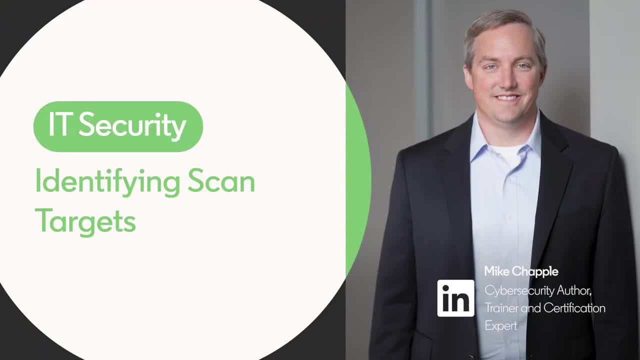 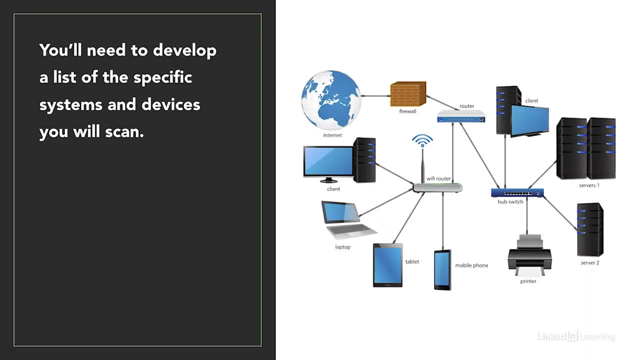 As you get a vulnerability management program underway, your first step is to develop requirements for that program. You'll think through whether the program is based upon a general desire to improve security, a response to regulatory requirements or a reaction to corporate policy. Once you've done that, your next step is to turn those general requirements 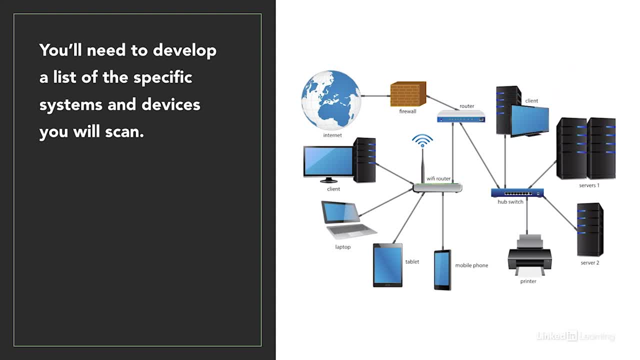 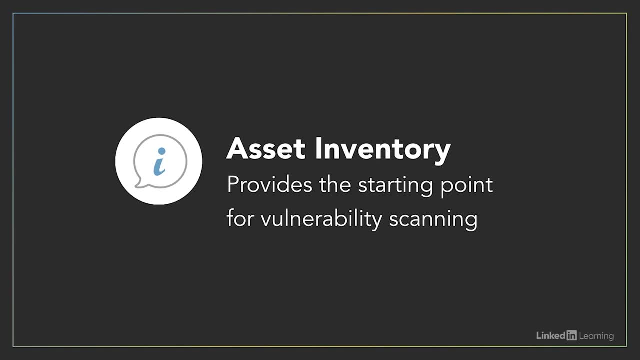 into a list of the specific systems and networks that you want to scan. In order to create this list, you need to have an asset inventory that you can trust. If your organization practices good asset management already, you may find that you already have this inventory ready to draw into. 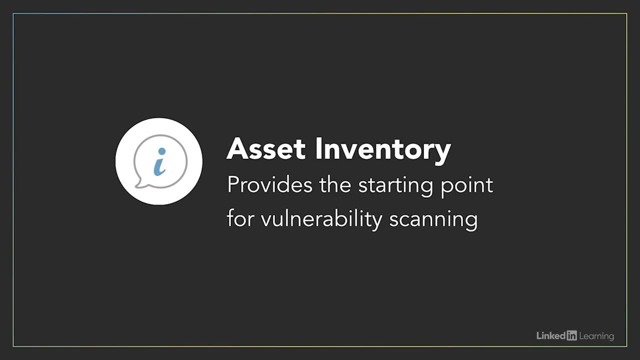 your vulnerability management program, You might find that your organization's configuration management tools already have a complete inventory of systems and devices on your network and, in the best case, that the inventory is kept up to date with information from regular network discovery scans. However, if you 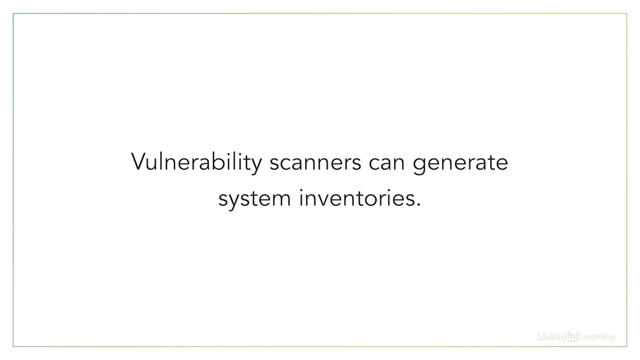 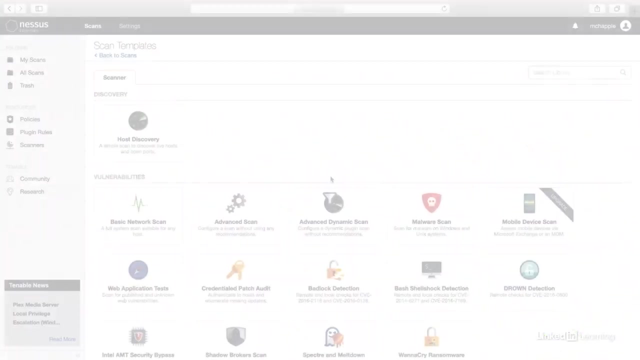 don't have this capability, you may instead turn to a scan run by your vulnerability management solution. Rather than running a full vulnerability scan, which can be very time-consuming, your system probably allows you to run a lightweight scan that just searches for systems on a local network. I'd like to show you how to set up a basic host discovery scan in Nessus. 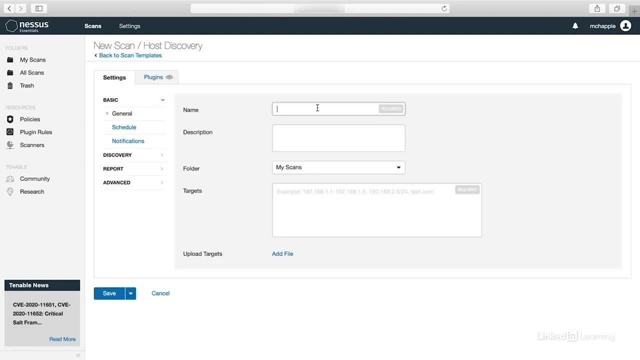 I'm just going to go ahead and click host discovery here, and then I'm going to give my scan a name- This is just arbitrary, anything that I'd like. I'll call it my internal network And then I can provide the scan targets and I'm going to use the private IP addresses of systems. 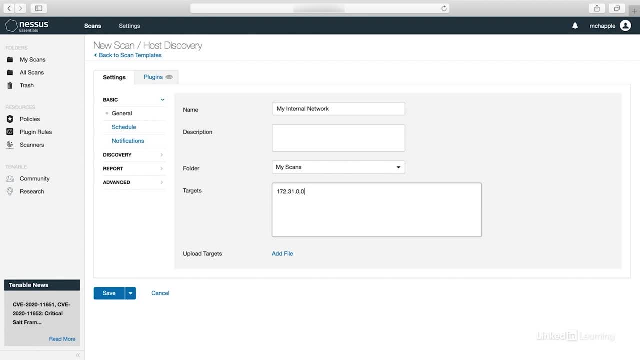 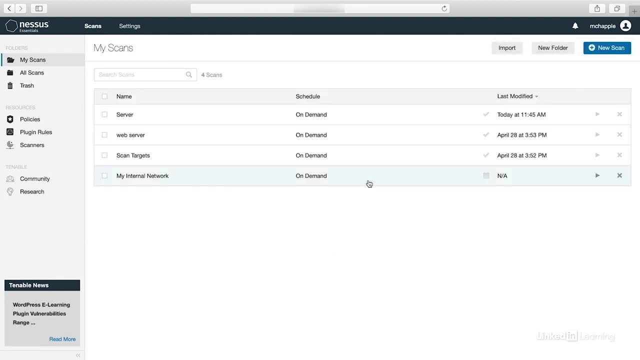 on this network, which is 172.31.0.0 slash 16.. Then I go ahead and click the save button and now, here in Nessus, I have my new scan and I can see that it hasn't yet been run. 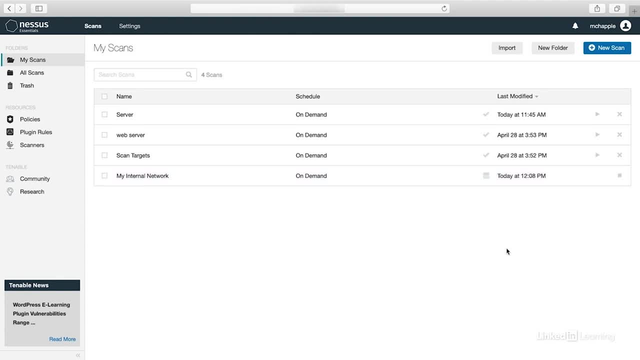 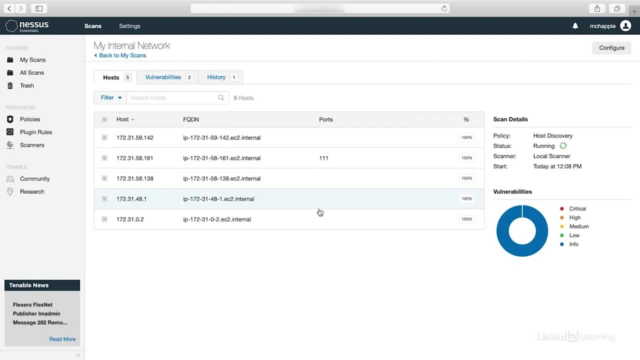 so I'm just going to hit this launch button here to launch the scan. Now the scan will start and take a little while until it finishes. As the scan runs, it populates a list of the hosts that appear on the network. These are hosts that I could then scan for additional vulnerabilities. 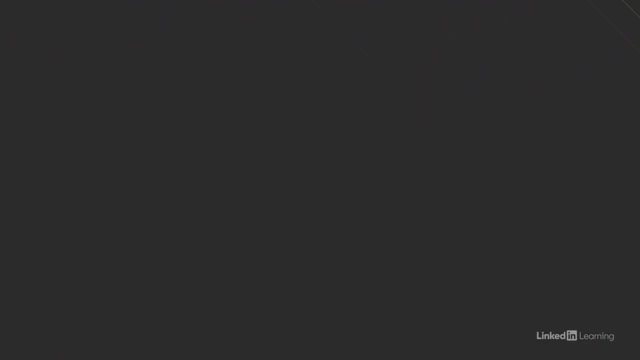 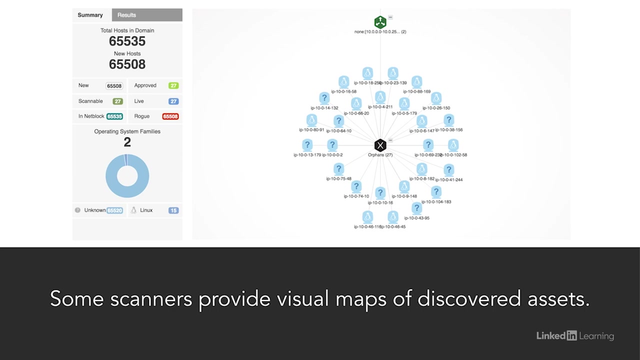 using more advanced vulnerability scans. Other scanners may also provide you with a graphic view of network discovery results. For example, here's a network map created with the Qualys vulnerability scanner. Once you have a solid asset inventory, you'll need to begin prioritizing those assets for your scans. This is normally done by answering.